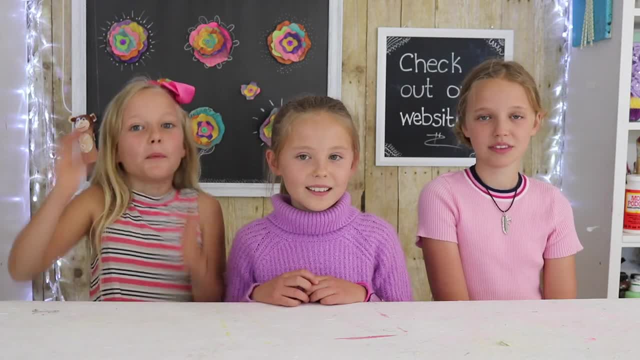 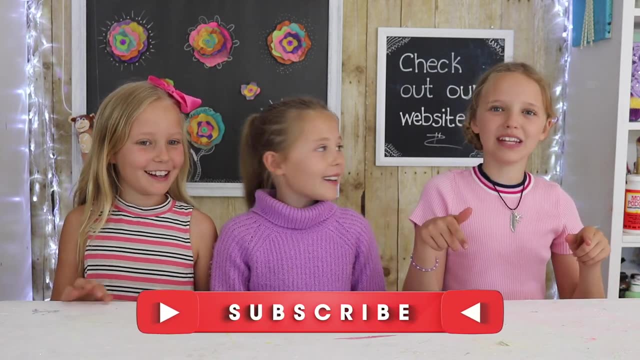 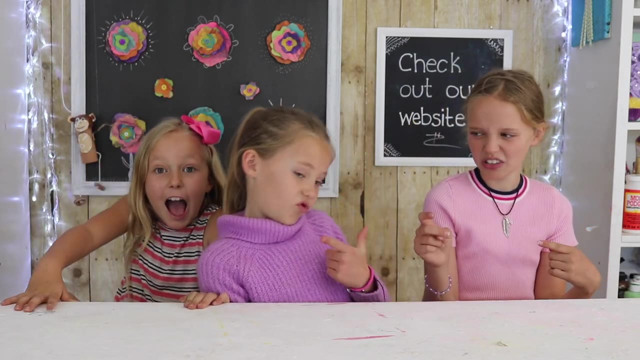 Today we're going to show you, guys, how we feed the birds, And then we're going to show you how we feed ourselves. Make sure to like, comment and subscribe For more videos in the future. make sure to hit that bell. Now on to the video And to make bird feeders. 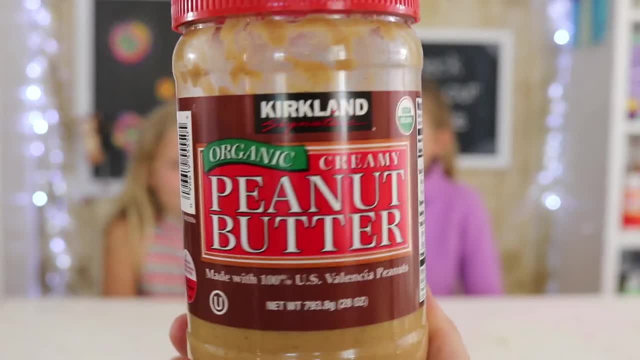 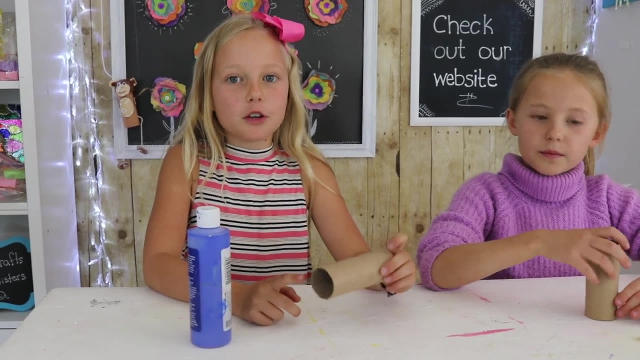 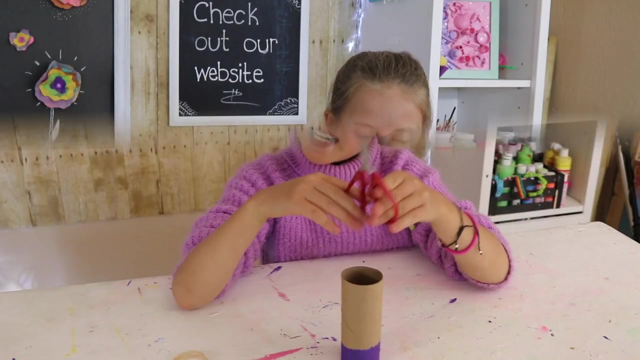 you'll need toilet paper rolls, peanut butter and sunflower seeds And string. The first step that you're going to do is you're going to paint the bottom of your toilet paper roll, so it'll add some color. The next step is to puncture two holes on the side of your 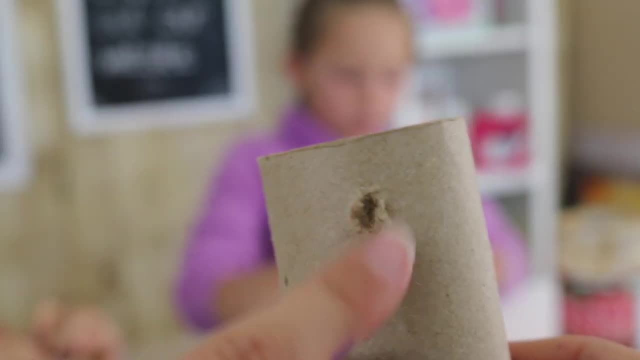 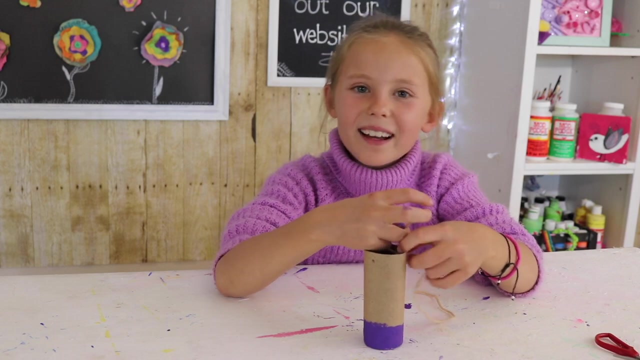 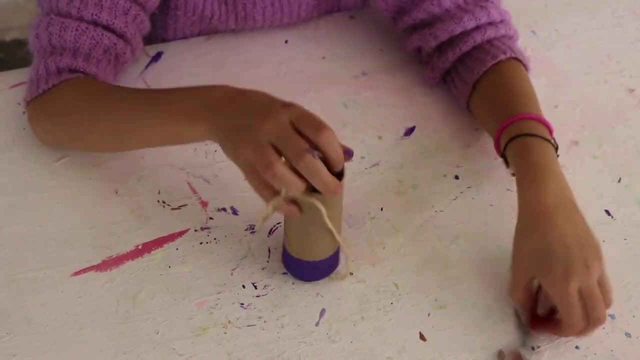 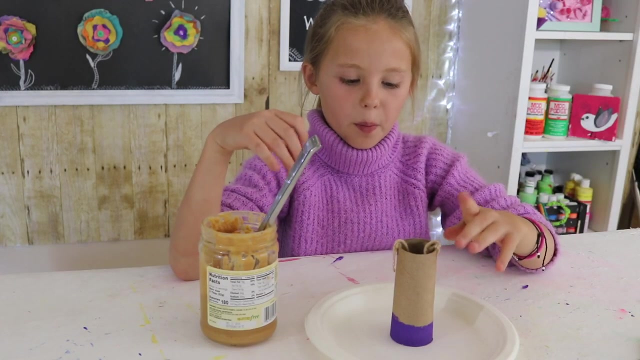 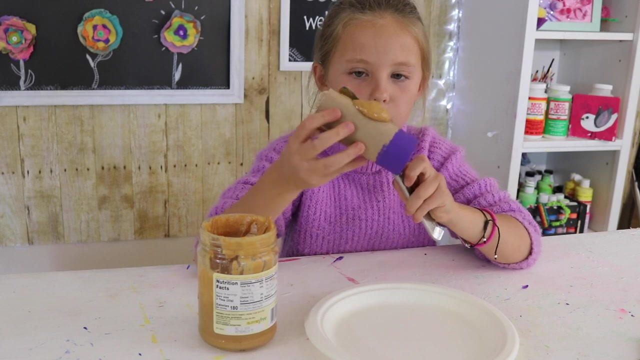 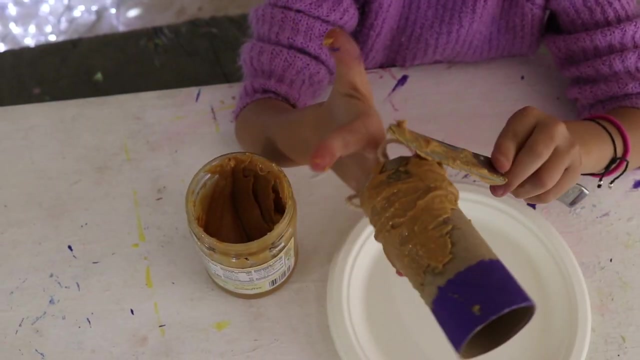 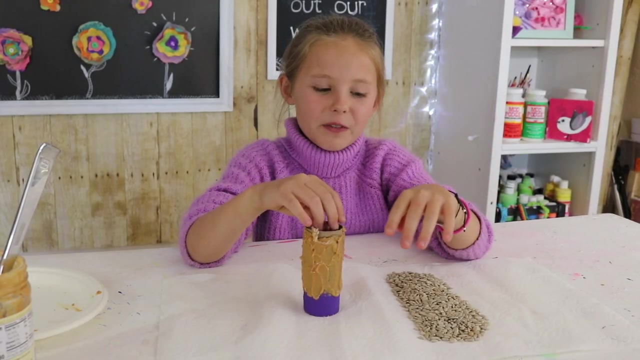 bird feeder. Now we're going to tie some string around the toilet paper roll so it can hang on the tree. The next step is to put peanut butter all over the bird feeder, except where you painted it. The final step is to roll the bird feeder in the seeds. 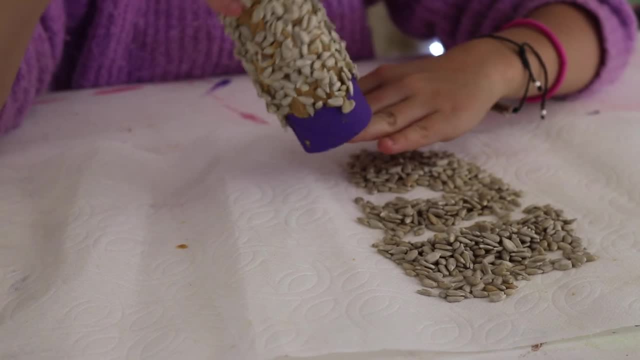 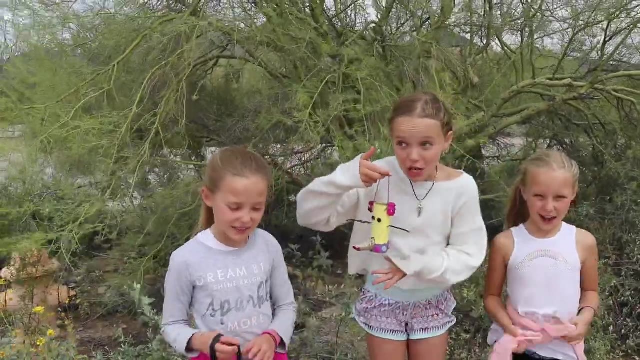 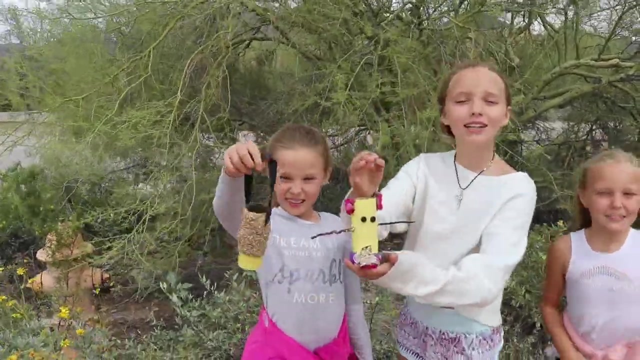 And this is the final result. Now we're going to go try these outside, Alright guys. so we've just finished our bird feeders and now we're at Gateway Trailhead and we're going to put our bird feeders up so the birds can eat some delicious ones. 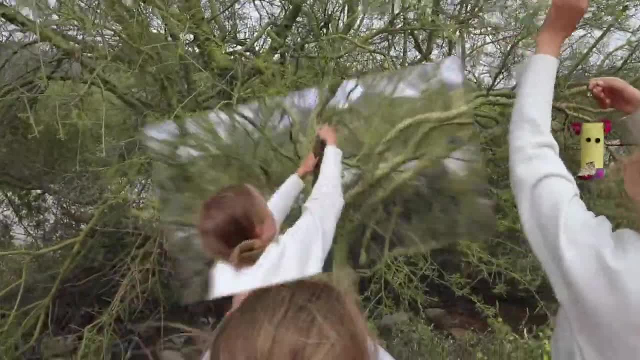 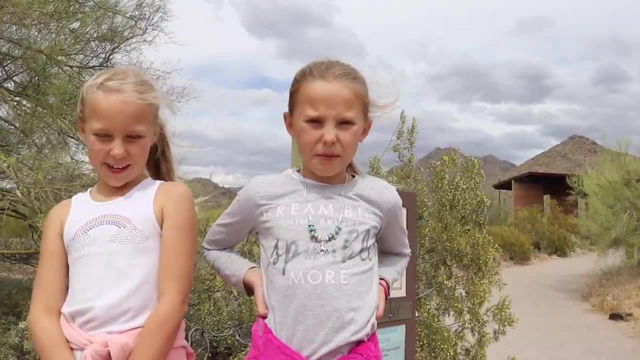 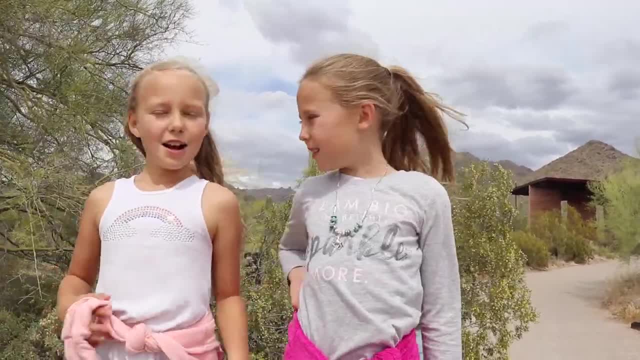 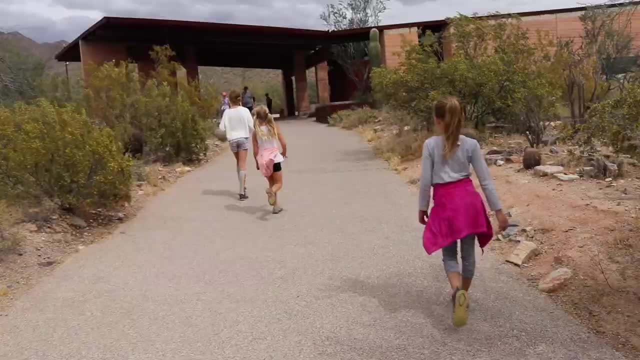 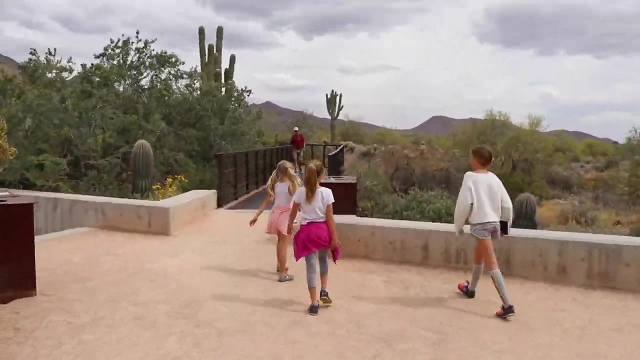 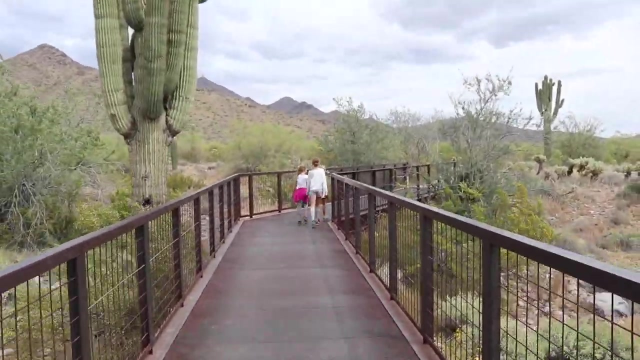 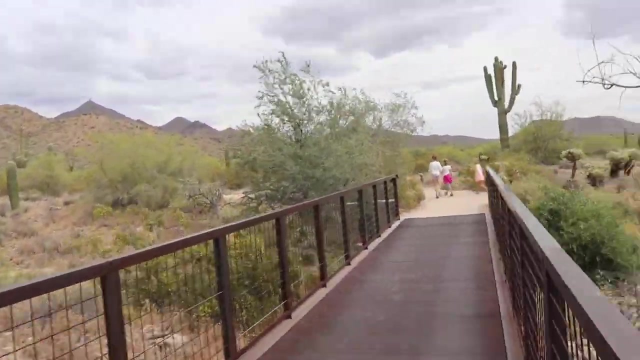 of Arizona, And we live in the state of Arizona. And we live in the state of Arizona And while we're waiting for birds to visit our bird feeder, we're going to go hike Gateway Trailhead. So let's go, Isn't that pretty guys? 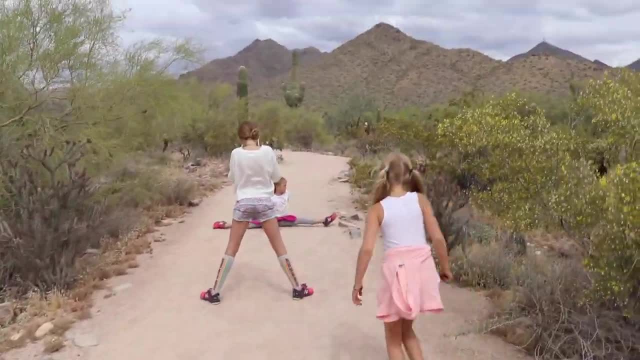 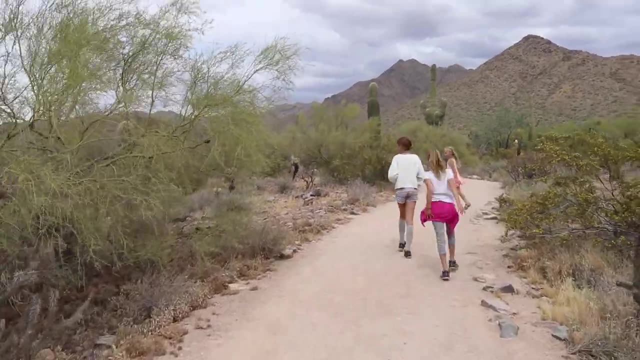 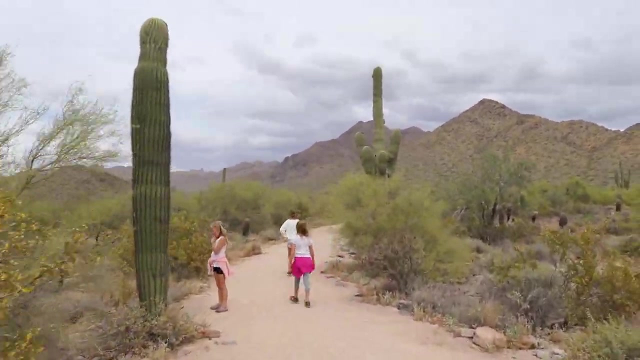 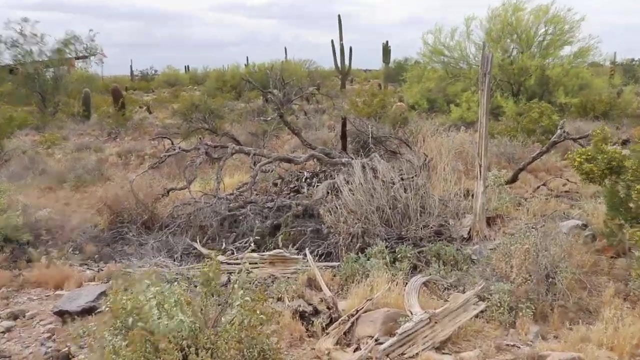 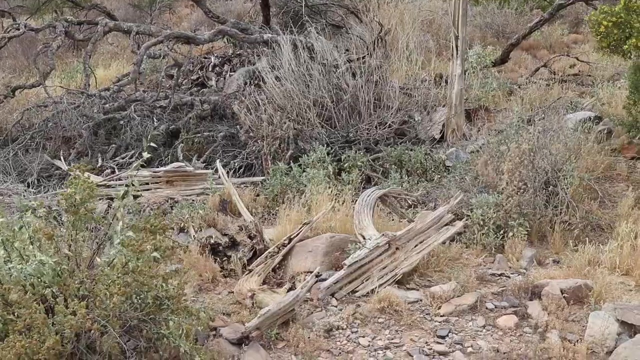 We're at the Calivari tree that probably got struck by lightning. That's a cactus that fell. I think it's a cactus that fell. It's a cactus that fell. Oh, my goodness, fell over. see the bones in the cactus. 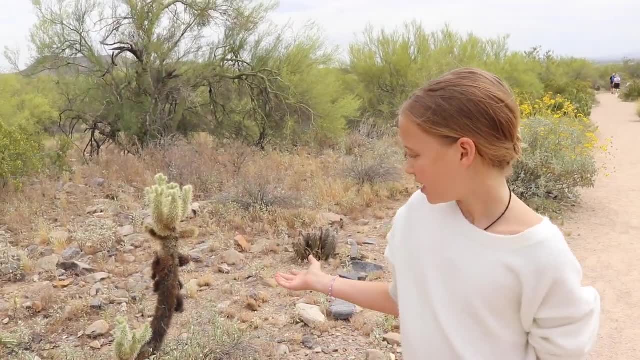 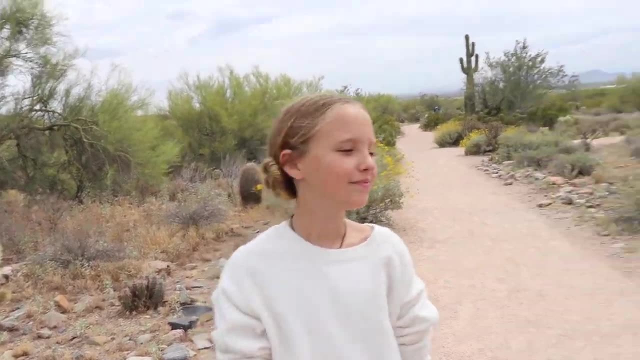 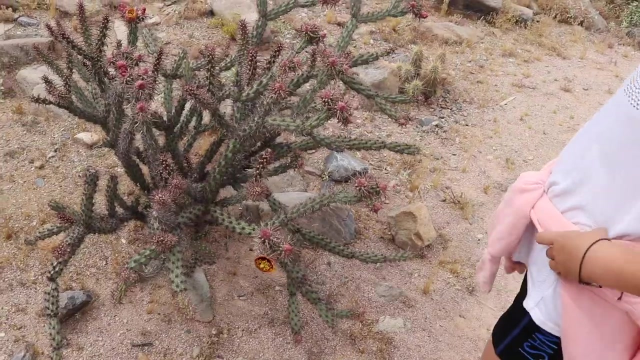 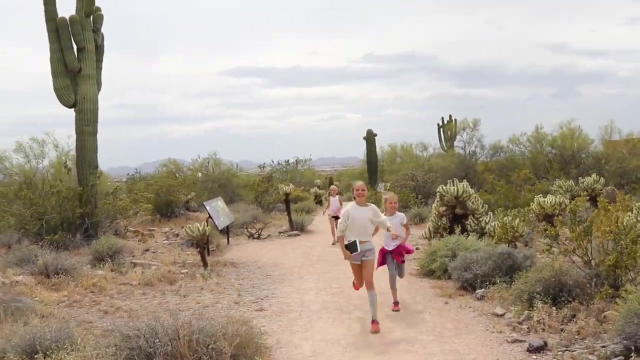 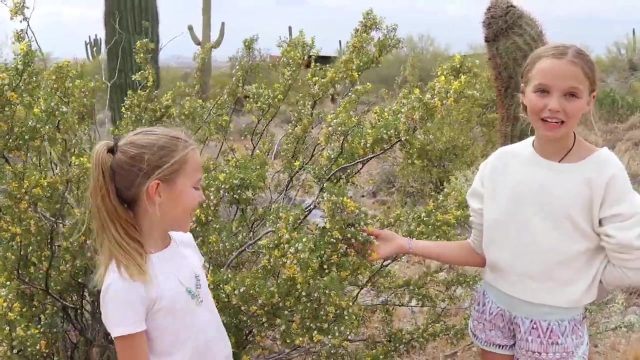 this kind of cactus is called the jumping cholla, so if one is on the ground and you walk too close to it, it'll jump onto your shoe or your your shin there. oh, it's warm. look at the flowers smell good. this is called a creosote bush, so when it rains it makes the state. 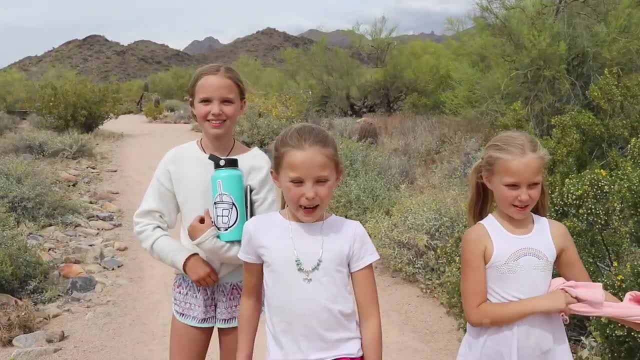 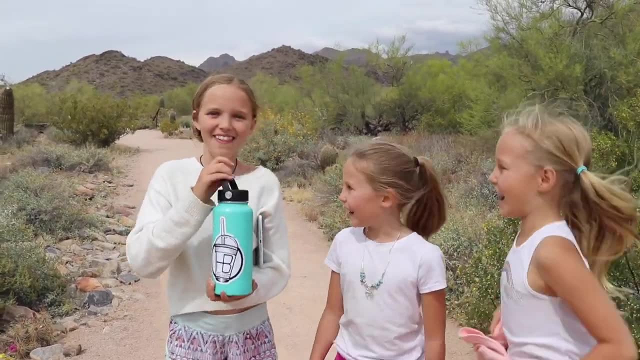 smell really nice. all right, guys, we've been hiking for about 45 minutes. now let's go back and check on our bird feeders. and what do you say about going to hb1? let's go, yeah, let's go. okay, guys, so now we're going to go check on our bird feeders and see. 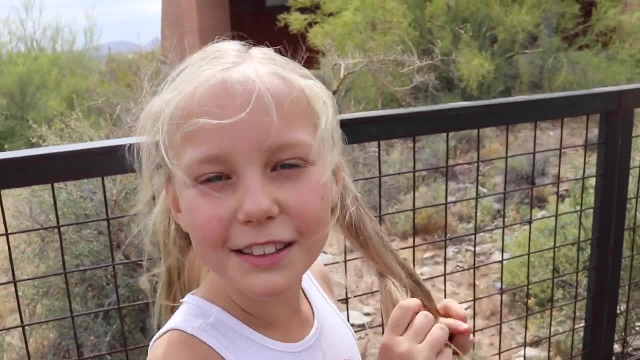 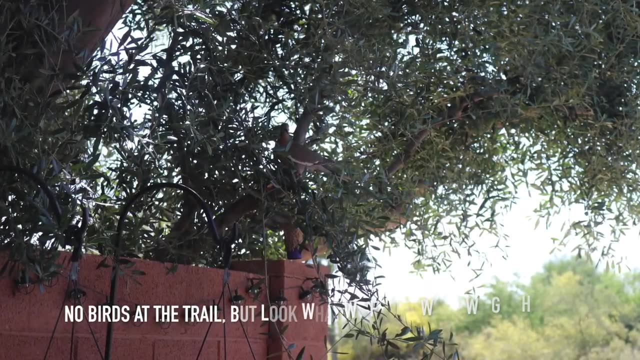 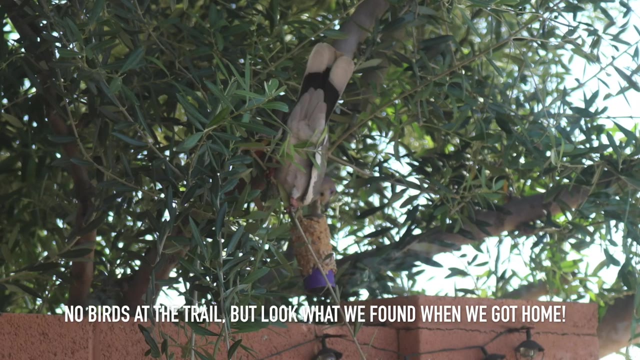 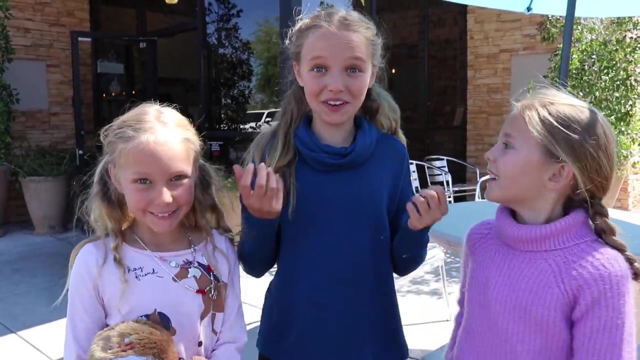 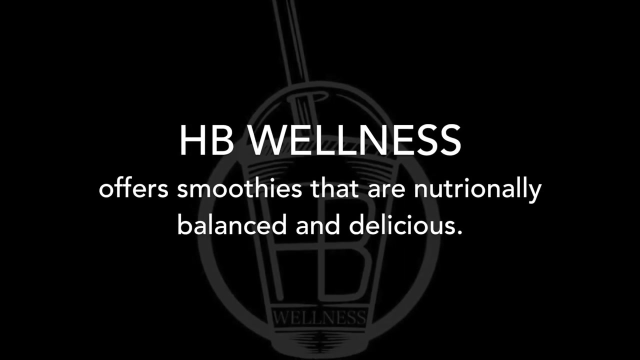 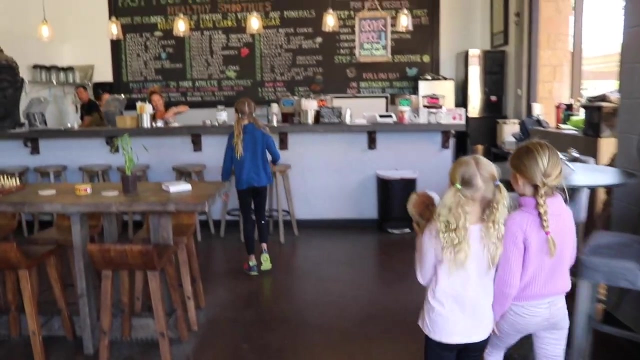 if any birdies have eaten our eaten our seeds. all right guys, so we're done with our hike and we're here at our favorite place- hb1 list- right guys? yeah, so let's go in and get a shake. good morning guys. hi guys, how are you? 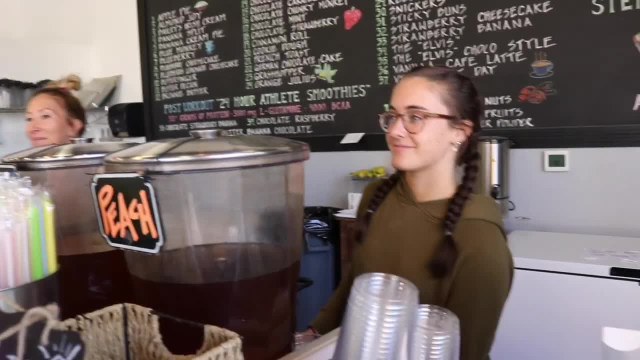 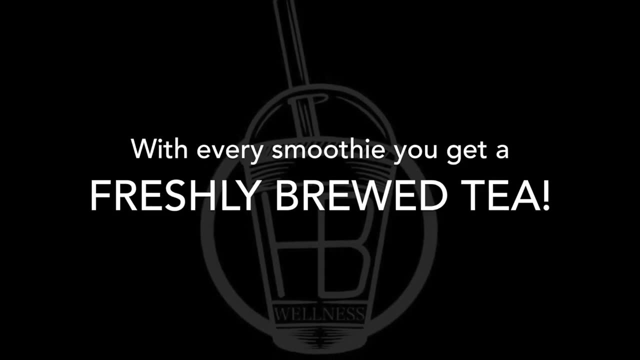 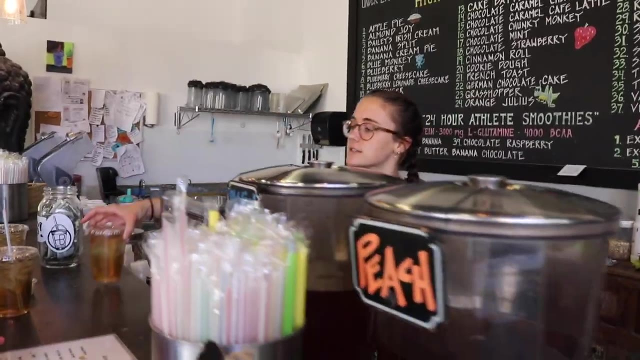 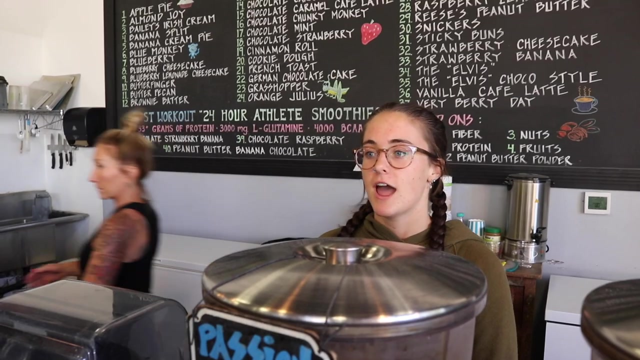 this is hannah. hi guys, this is hannah. hi guys, this is hannah. this is hannah. so what's so important about the tea? so all the teas are green tea based um. green tea helps you boost your metabolism, burn roughly 90 to 120 calories, and it's also sweetened with aloe vera and the 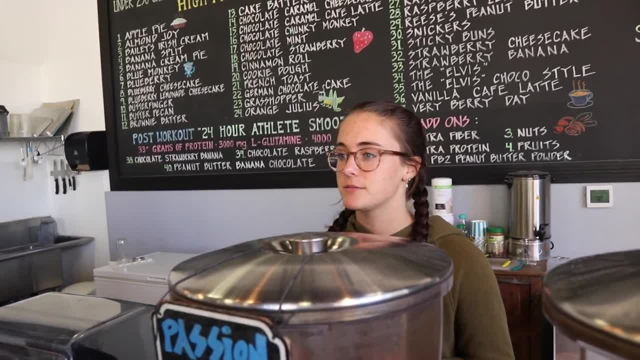 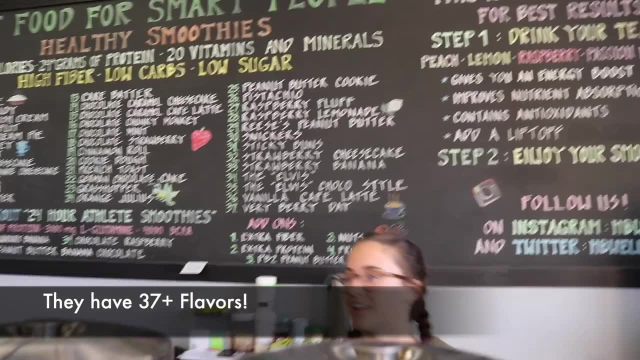 aloe vera helps you digest everything better in the shapes. it's good for your gut and helps everything move along nicely. yeah, look at all the flavors they have. they have a secret menu too. yeah, and this is the secret menu. that's what i've ever said. all right, girls, let's use today. 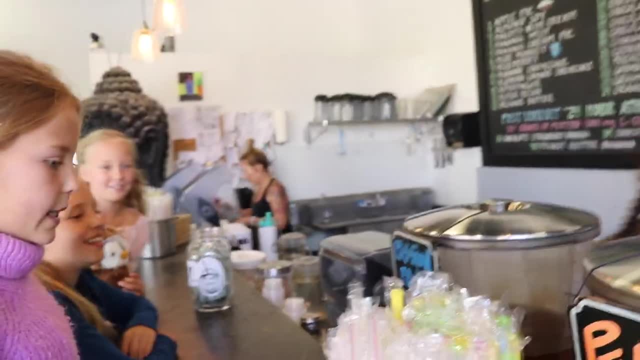 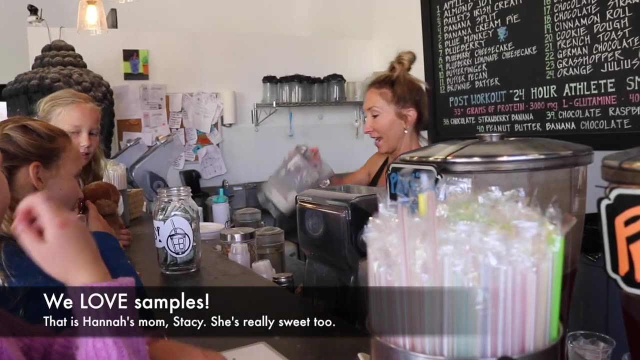 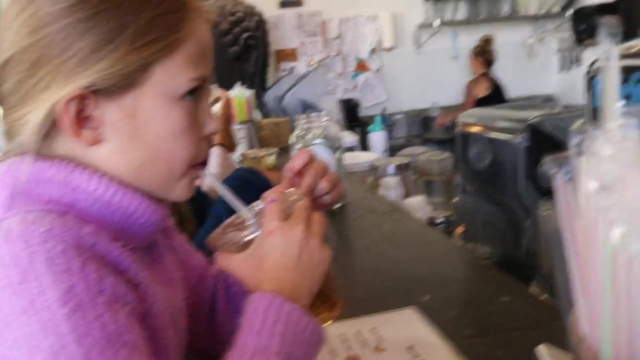 um, three pieces, three pieces, all right, and i'm going to give you some samples today. this is banana bread. i don't think you guys have ever had this one, no, but they're good. here's one of those. thank you, you're welcome. uh, pina colada please. 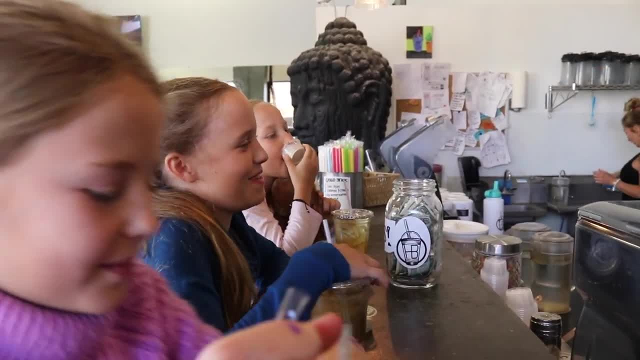 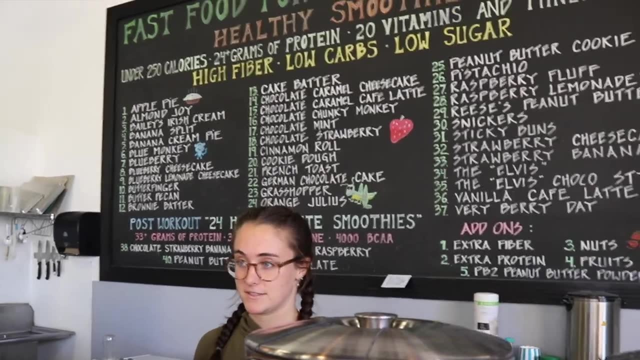 pina colada. okay, we're just going to use three pina coladas, all right. what's the most popular shake? all right, we have a coffee. we have a couple that are amazing. most of them are amazing, but some of the top ones are birthday cake, banana cream pie. sugar cookie, coffee ice cream, vanilla, magic bar, mint ice cream, and i know it sounds like they're unhealthy because it says ice cream in them, but they're all under 250 calories, 24 grams of protein. there's no ice cream in it, it's just water and ice paste. 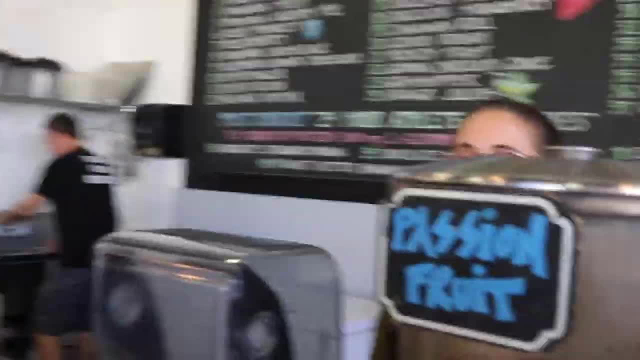 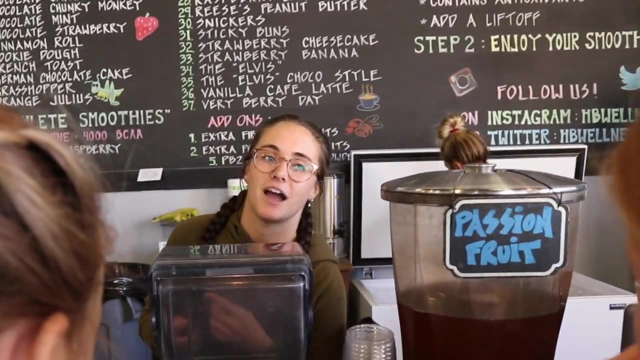 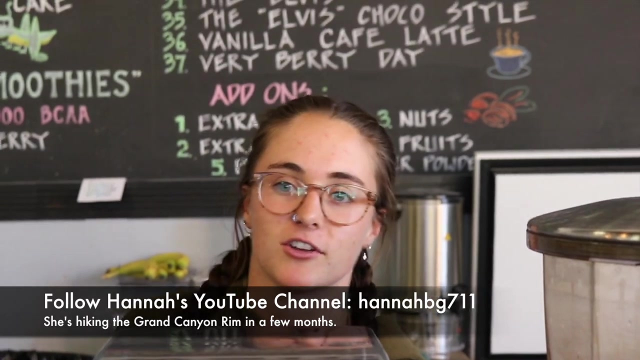 yeah, that makes her mom happy. what's your favorite shake? that's hard for me. i like oaklawn, but some of my favorites are sugar sugar cookie, because i made that shake so i'm a little biased by that. but um, that one and birthday cake and banana cream pie are honestly some of my favorites. 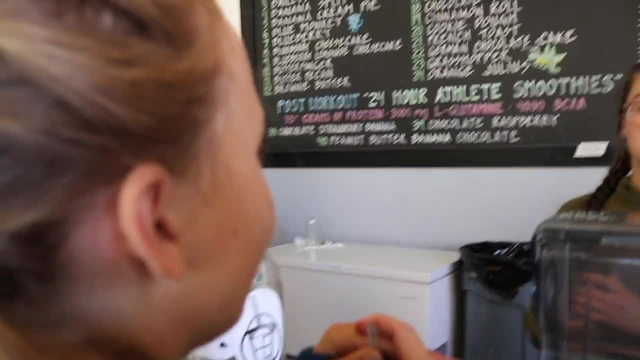 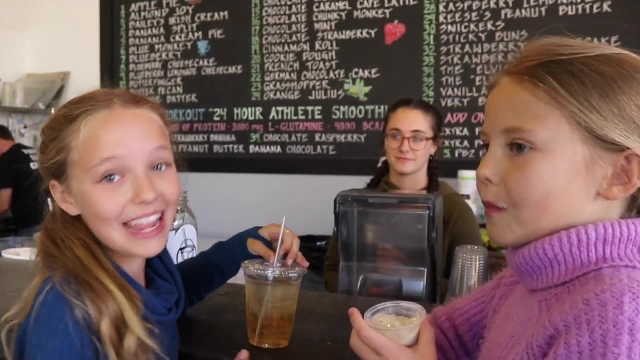 and is hb wellness just in arizona or nationwide? this is our only location that we have, yet so it's only located in arizona. so, guys, if you're here in scottsdale, you'll have to stop by hb wellness. the address will be in the link in the description box below. 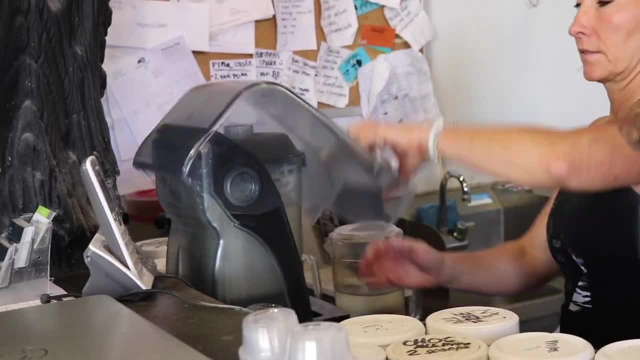 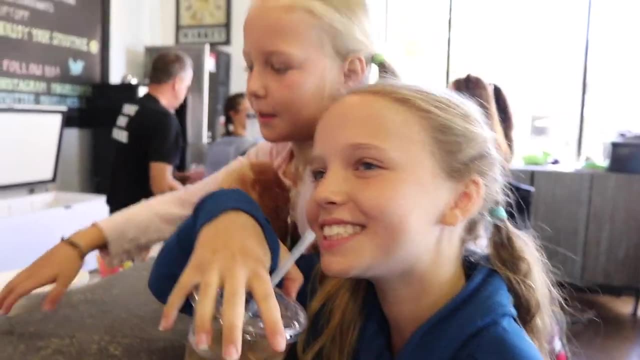 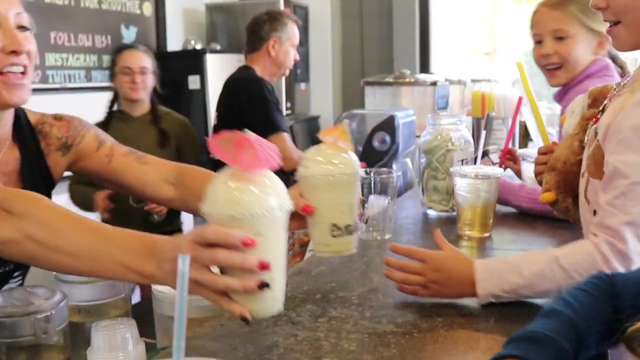 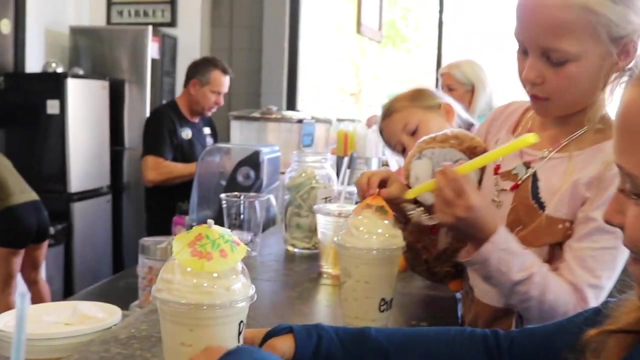 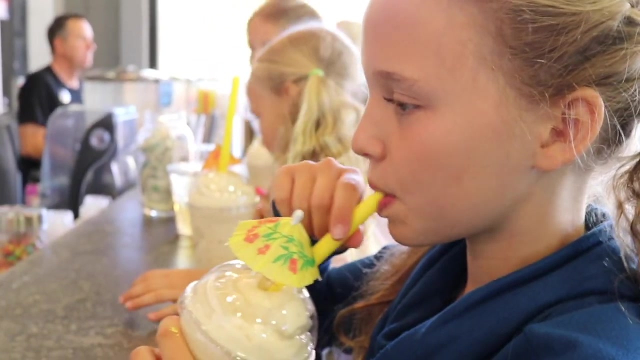 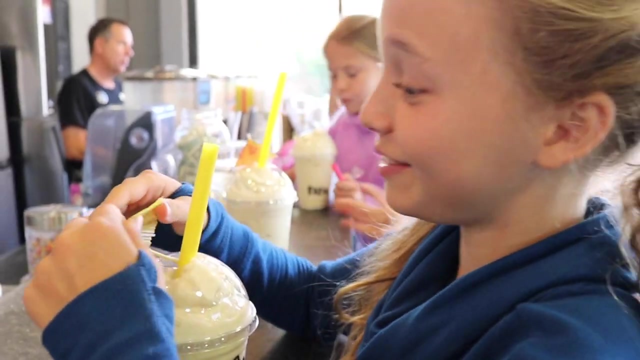 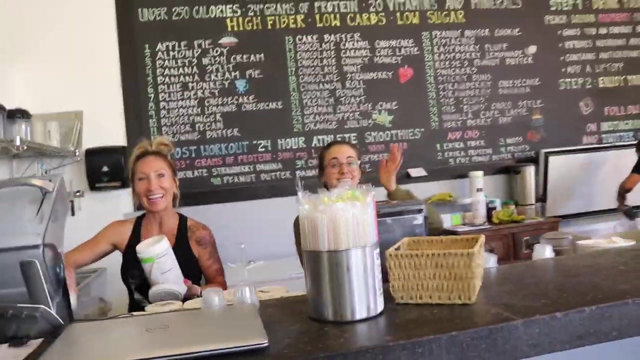 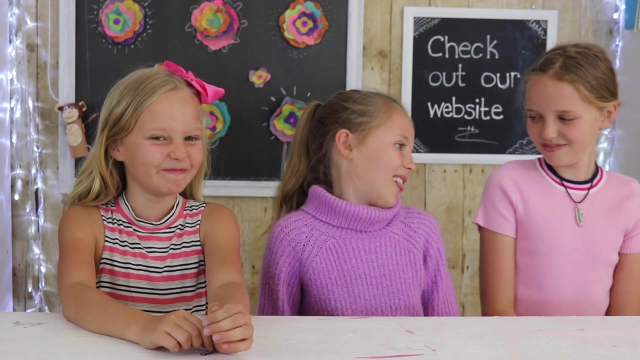 i normally get birthday cake, but i'm kidding that pina colada is new, so i'm going to try. there you go, thank you, you're welcome, enjoy. thanks, and it's good for you and i love that. happy birthday, sweetheart. thank you, give me a test.